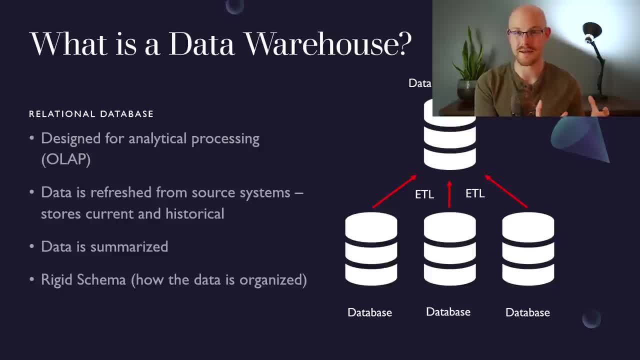 need Now. a data warehouse is also a database, just like we were looking at before, but it's going to be used for analytical processing, or OLAP. OLAP stands for online analytical processing and it's created to basically analyze huge amounts of data. Now, if you notice, on the last slide, 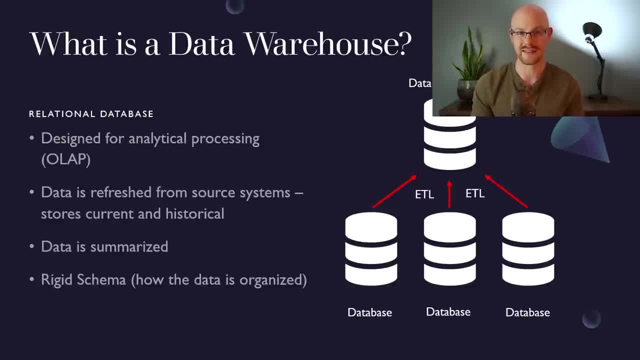 there were these three databases and they were just kind of sitting there and they were storing the data In this visualization that we have on the right. these three databases on the bottom are all aggregating and sending their data to this data warehouse via an ETL process, which is where 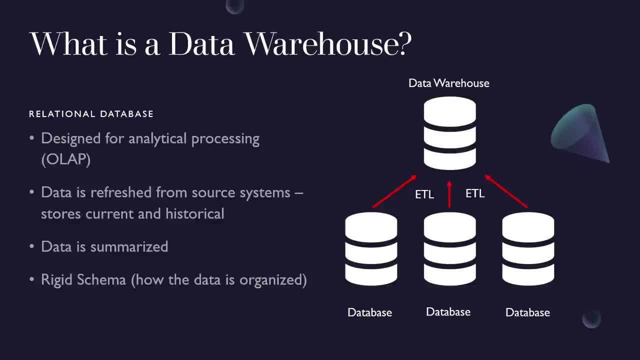 it extracts the data, it transforms it and loads it, exactly how they need it, in this data warehouse. And that's how data is put into the data warehouse. It isn't getting it directly from the source, but it's being put into a database and, via the ETL process, it's being updated as it goes, or 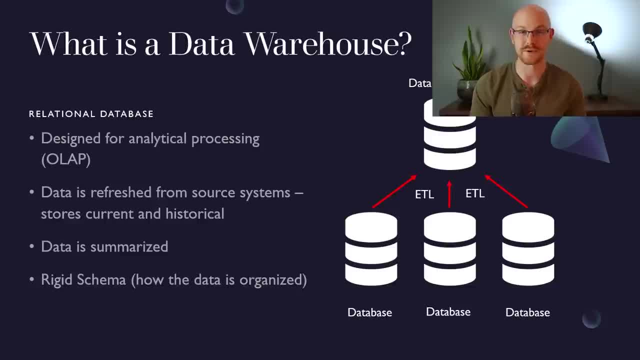 whenever the ETL process runs, The data warehouse will always have the historical data, but it won't always have the current data, unless the ETL process is running every single day or very frequently. The data in the data warehouse is also a little bit different because we're doing this ETL process to get the data in. 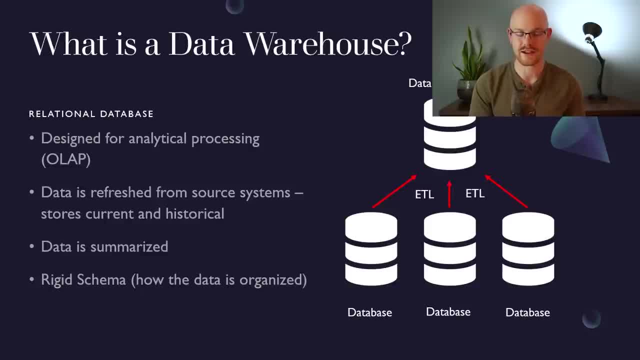 there. We're not actually putting every single piece of data or every column and row in there. We're typically summarizing it and then putting it in there, which will allow us to process that data for our analytical purposes much faster. Now a data warehouse is going to have a much 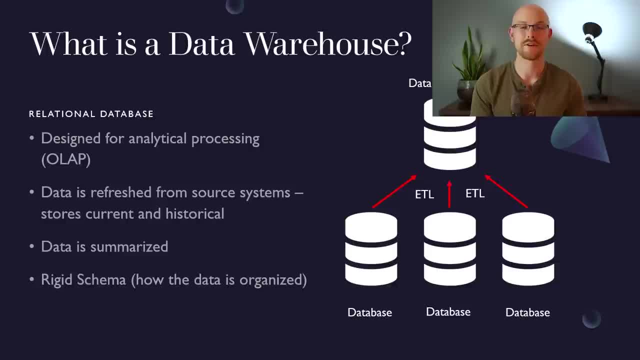 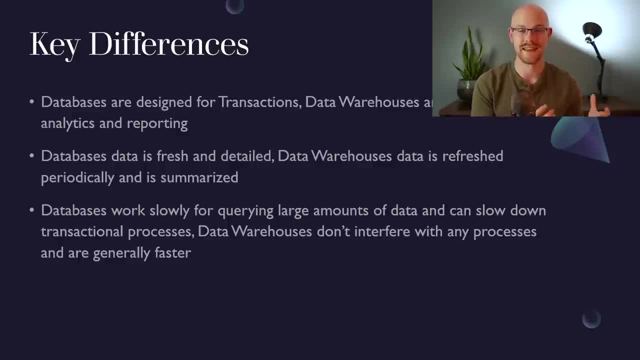 more rigid schema, so you really need to plan ahead With how you're going to put your data into a data warehouse. it's not as flexible as just a database, So now let's look at some of the key differences between a database and a data. 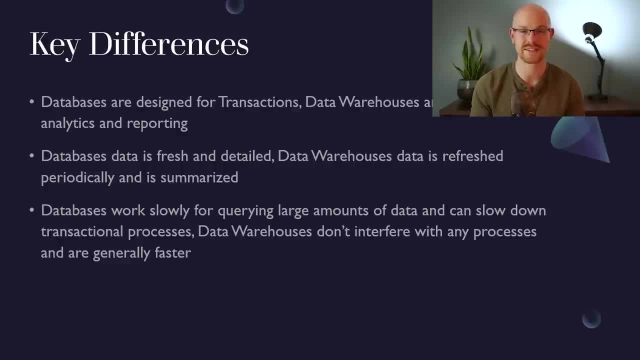 warehouse. A database is going to be used for recording transactions or a data warehouse is going to be used for analytics and reporting. A database is going to have fresh and detailed data. where a data warehouse is going to have summarized data, It's only going to be as fresh as the ETL. 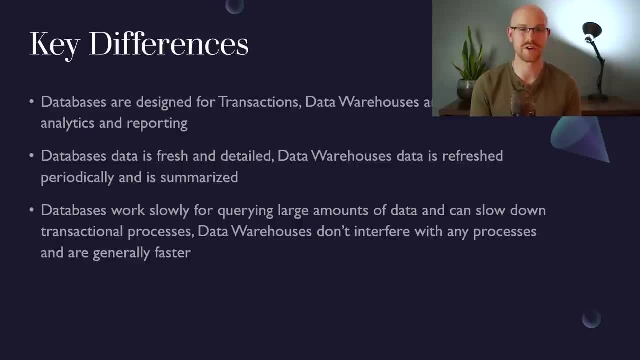 process is created. A database is going to be a little bit slower for querying large amounts of data. And when you do query large amounts of data, it's going to be a little bit slower for querying large amounts of data. It can actually slow down the processing of all those transactions. A data 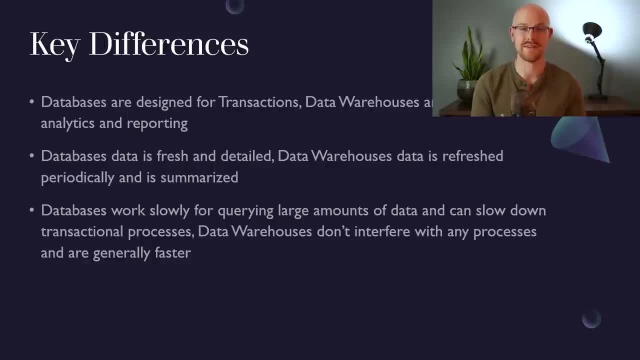 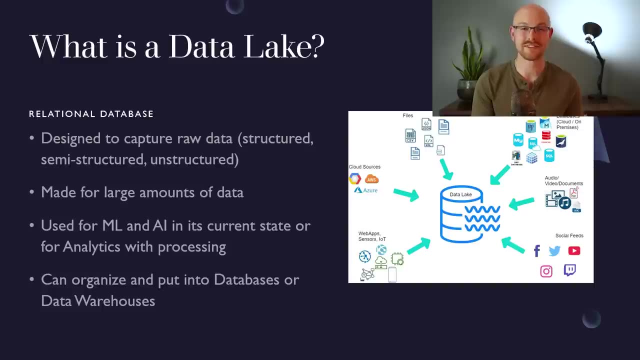 warehouse was designed for the exact opposite. It was designed to be very fast at querying and not slow down any processes, because it isn't part of that transaction processing at all. So now that we've looked at a database and a data warehouse, let's take a look at a data lake. A data lake was 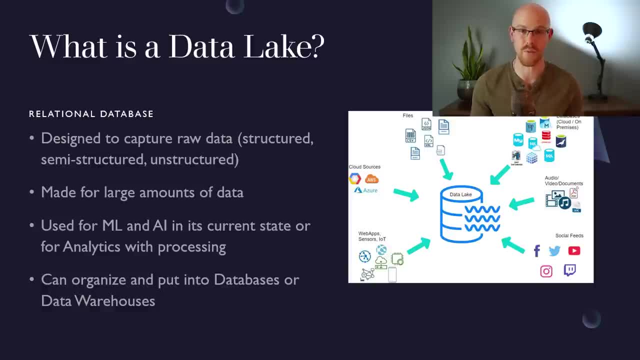 basically designed to capture any type of data that you could possibly want. It could be a video, a picture, an image, a document, a graph- anything you could imagine that you'd want to put in a database or store. in some way You can store it in a data lake. Now there are a ton. 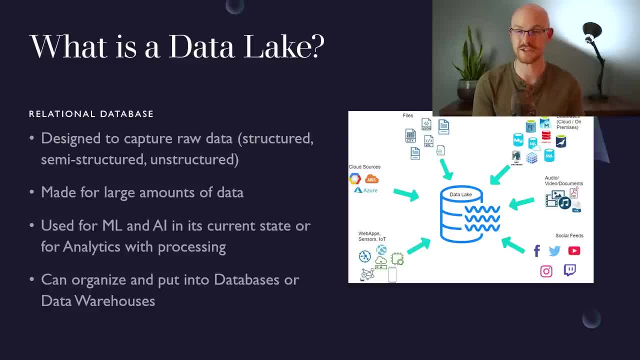 of use cases for a data lake, but I think people who work with machine learning and AI get to use it or benefit from it the most. They can use all that structured and unstructured data and create models to really use it in its raw form, where, if you want to use it for analytical purposes- 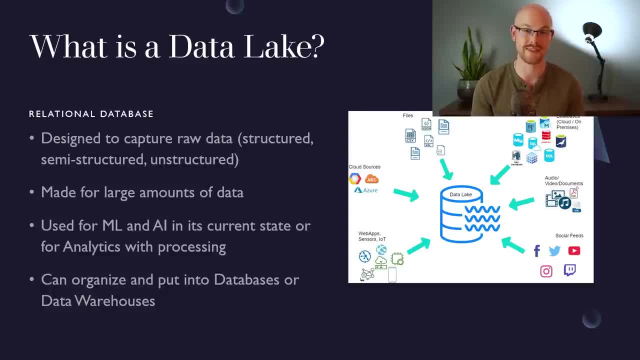 typically, you're going to have to clean it up a little bit and do a little bit more work to actually make it usable, And so a data lake is just that. It's this lake where you can basically throw any type of data in there, but it's not going to be a data lake. It's going to be a data lake. 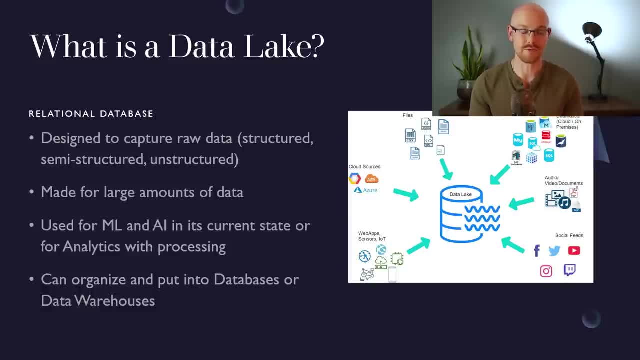 It's not always super usable because you're just putting it in there in its raw form. If you want to use it for analytical purposes and reporting, most of the time you're going to want to clean that up and put it into a database or a data warehouse. So now, when we're looking at all three, 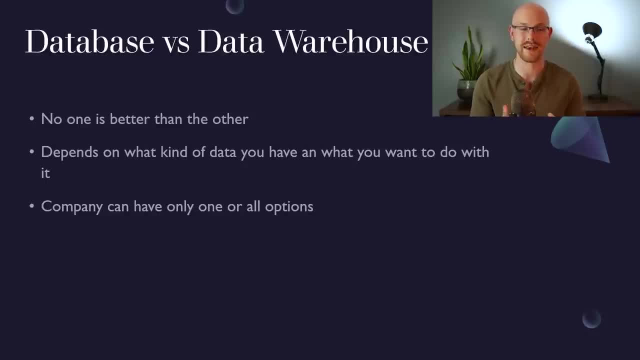 they are all different and they're all used for different purposes, So no one option is better than another for your data. If you're using it just to record transactions, a database is what you should do, And if you have a large amount of data, that's just too much for your database to. 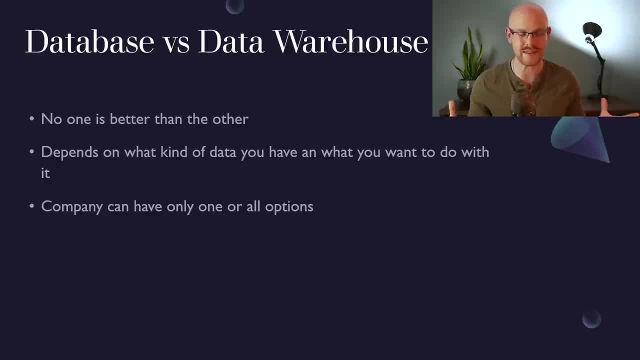 handle. it sounds like you might need a data warehouse, And if you have all this data, you're going to want to use it for analytical purposes. So if you're using it just data, they have no idea what to do with, or it's unstructured, it's semi-structured data that you 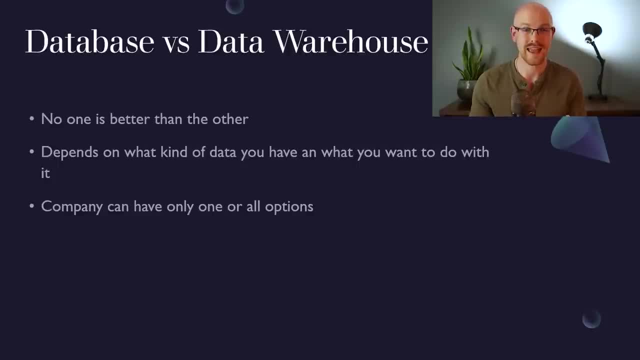 can't fit into a database, Well then, I highly recommend using a data lake. There really is no one size fits all. All three of these can be options for different uses And in fact, you can use all three within one company for just different things that your company needs. So I hope that.